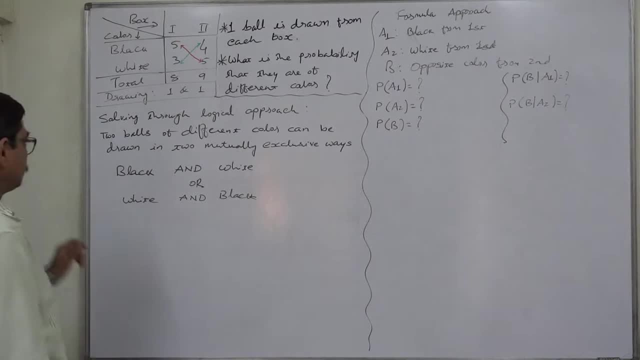 through logical approach, No formula, no sign we are going to use, And that is: two balls of different color can be drawn in two mutually exclusive ways. That is, two balls of different color can be drawn in two mutually exclusive ways. That is, two balls of different. 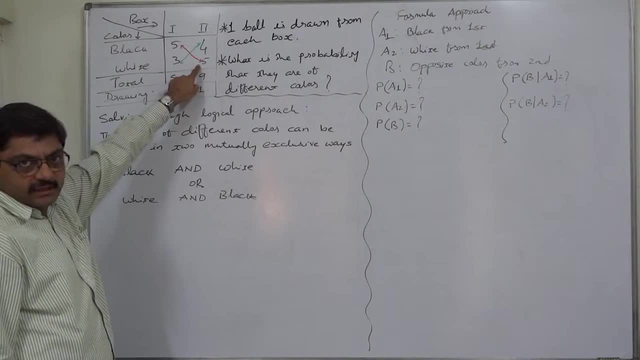 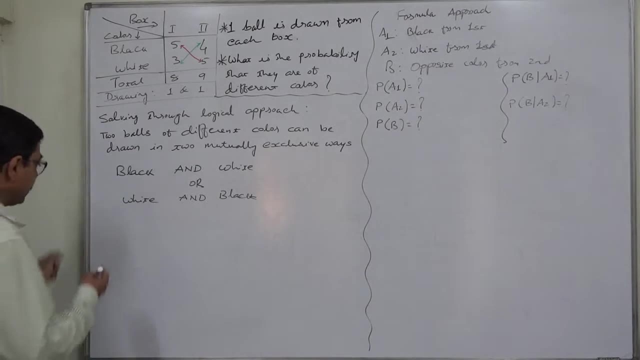 color can be drawn in two mutually exclusive ways. Now we will use this method. The process is black from first box and white from the second, Or white from the first box and black from the second. Let us calculate probability of this event Required. 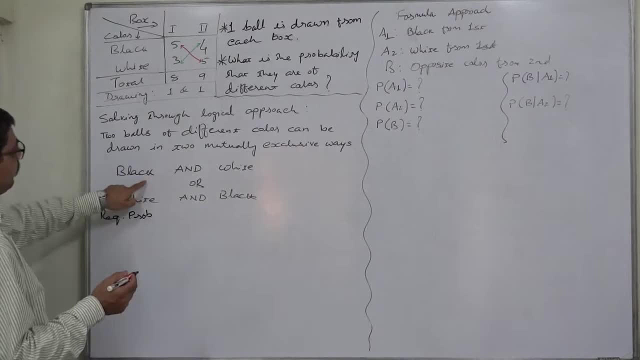 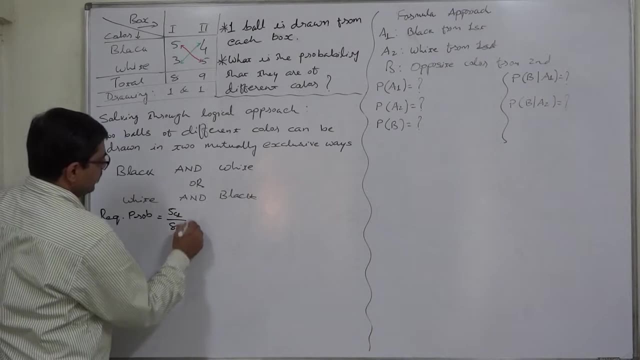 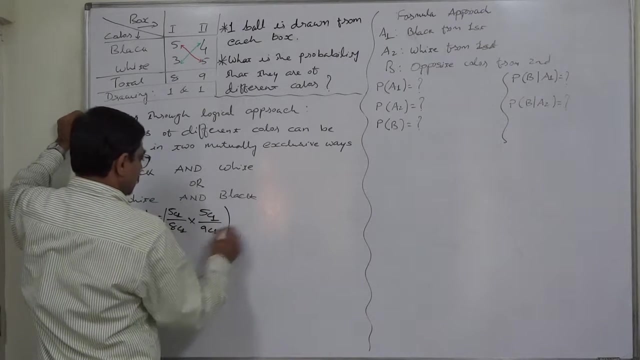 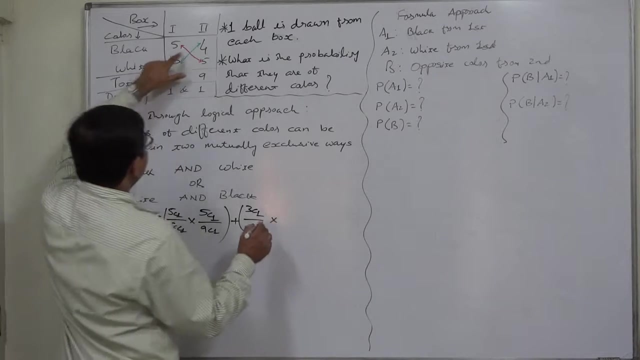 probability or probability of this event is black from the first box, That is, 5 c 1 upon 8 c, 1.. And white from the second, 5 c 1 upon 9 c. or white from the first, 3C1 upon 8C1, and black from the second, 4C1 upon 9C1, just. 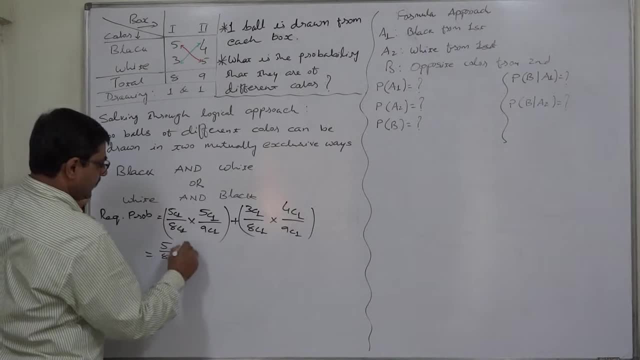 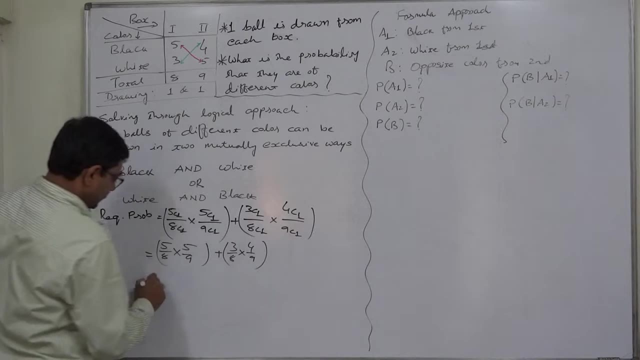 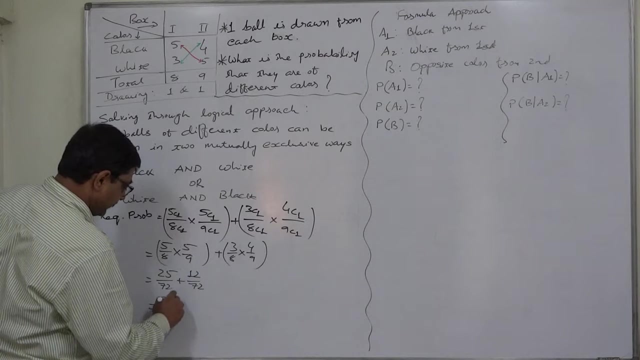 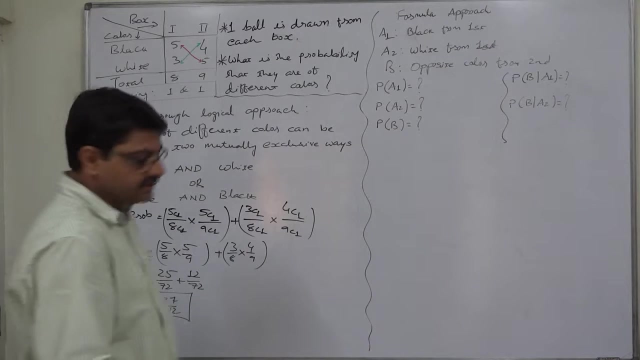 simplification: 5 by 8 into 5 by 9, plus 3 by 8 into 4 by 9, and that is 25 by 72 plus 12 by 72, that is 37 by 72. now let us solve this problem through formula assigning the various signs to: 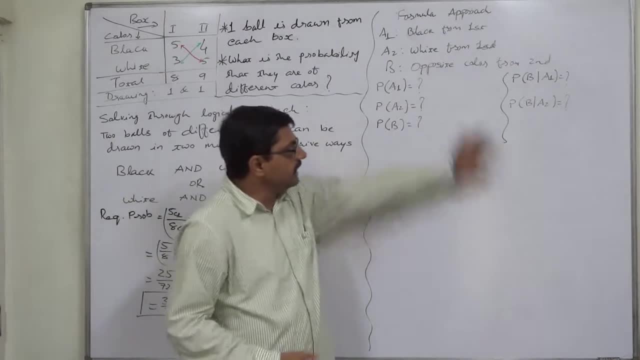 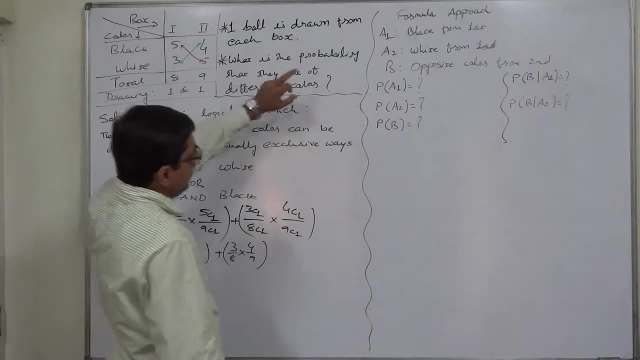 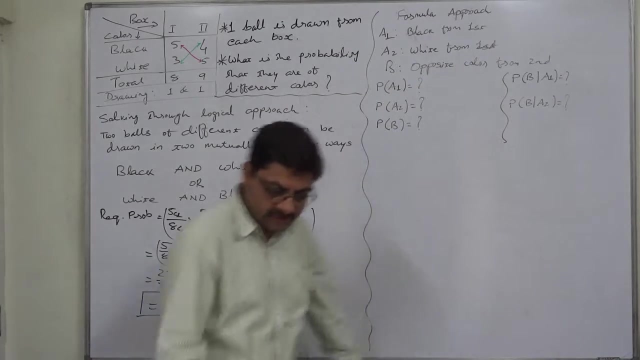 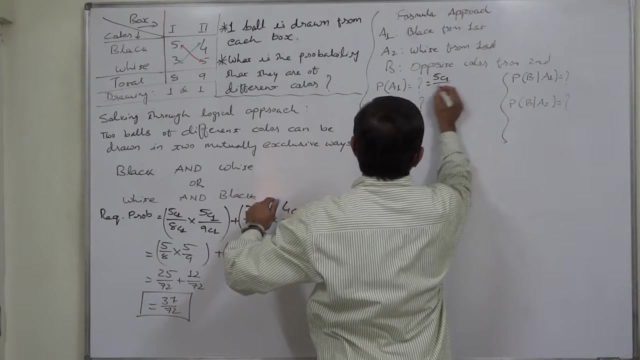 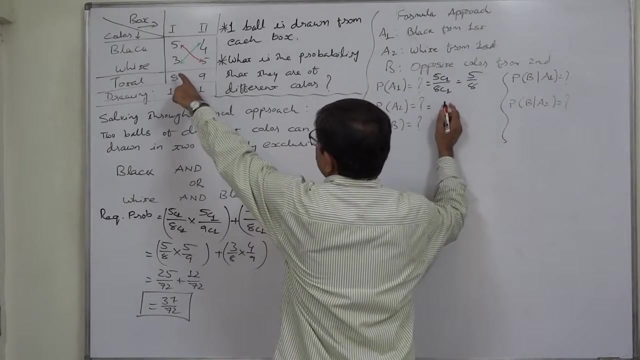 probability, etc. you will observe that this one is a longer process. first of all we have to use sign a. one is black from the first box a. two is white from the first box. B is opposite color from the second. now, P of A1: black from the first, 5C1 upon 8C1, that is, 5 by 8. P of A2: white from the first, that is 3C1. 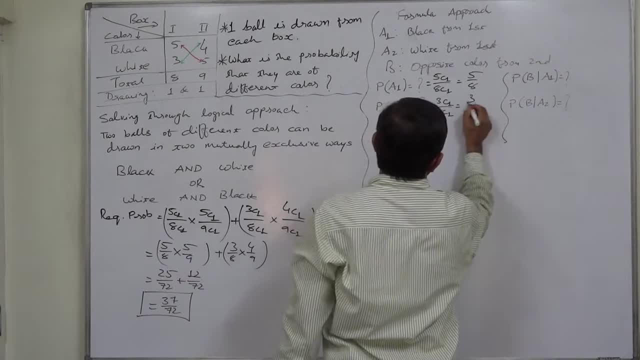 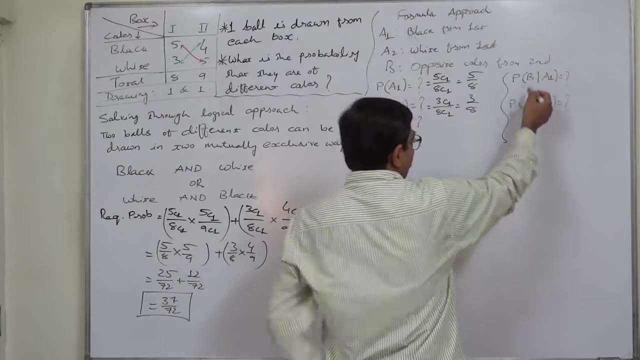 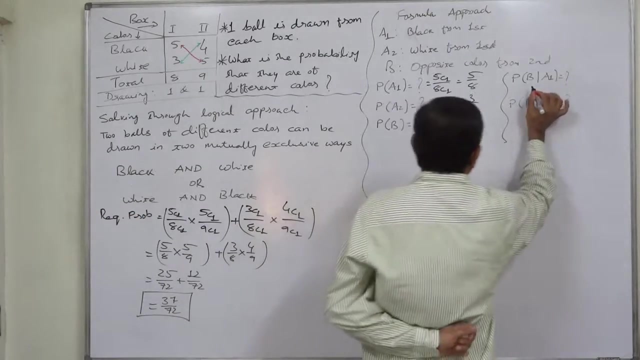 upon 8C1, that is, 3 by 8. P of B is not possible at this stage because ball of different color is dependent on the color of the ball in the first row. so if in the first row we help drunk like, in the second it will. 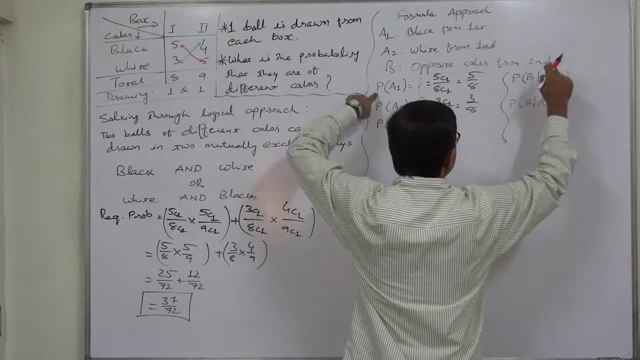 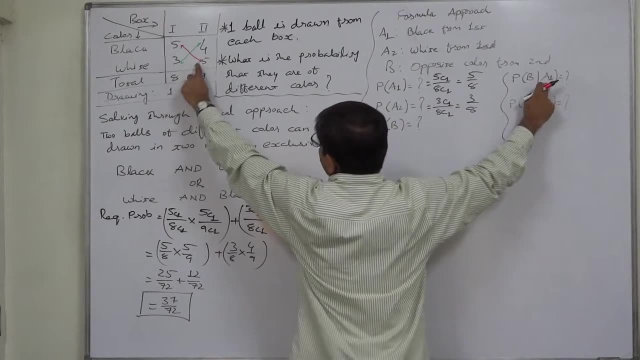 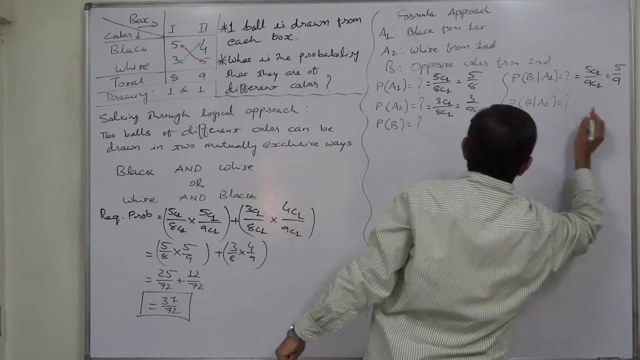 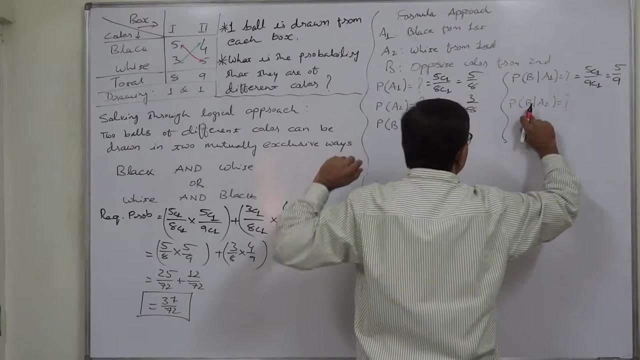 divide. so probability of white in the second row if a blake was drawn in the first row, that is, white in the line from the second. five c1 upon 9 C. well, that is five by nine. similarly, probability of being given A2 will be probability of black from the second. If white was from the first, black from the. 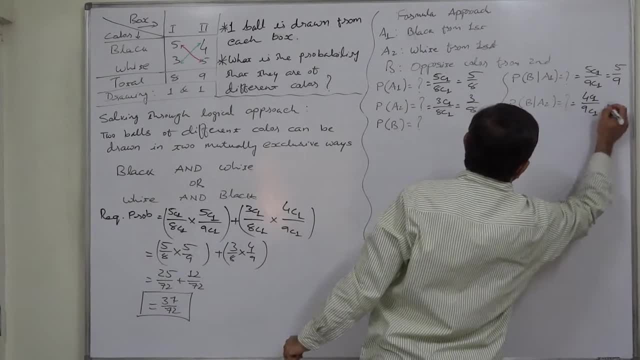 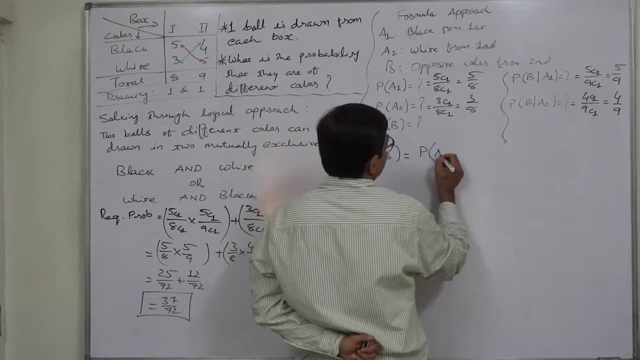 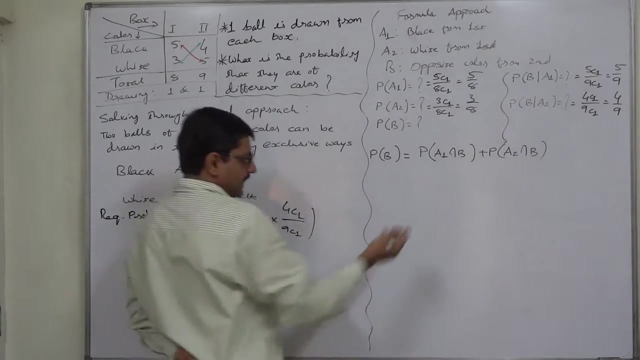 second, 4C1 upon 9C1, that is 4 by 9.. Now P of B is possible in two mutually exclusive ways: P of A1, intersection B, plus P of A2, intersection B. Now we are well aware that 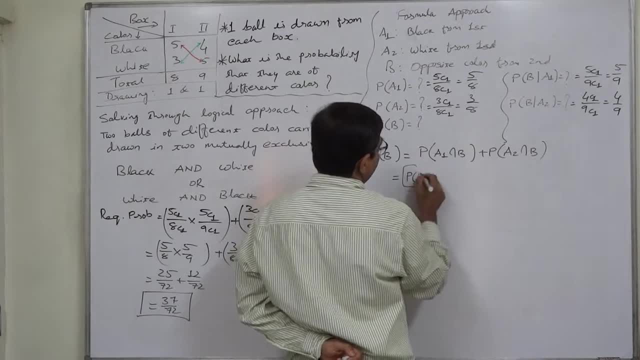 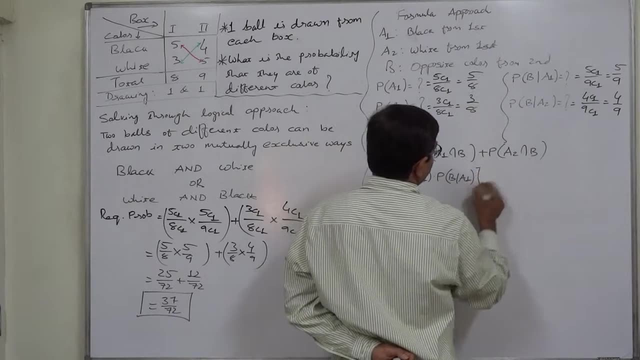 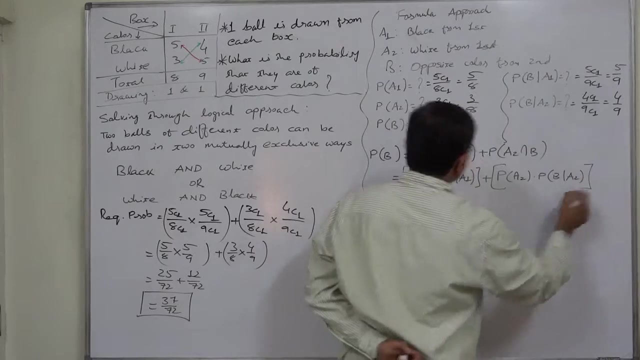 this is possible through the formula P of A1 multiplication law we are going to use into P of B given A1, plus P of A2. into P of B, given A2.. P of A1 is 5 by 8. into P of B given A1. 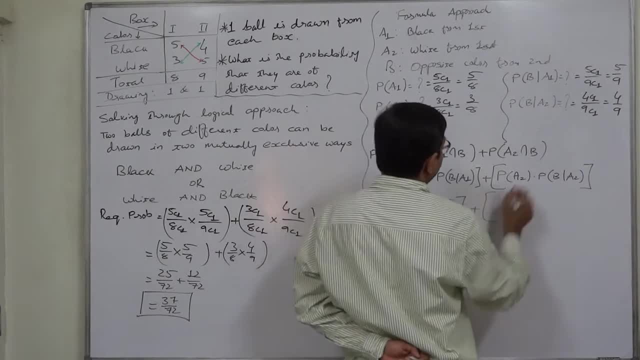 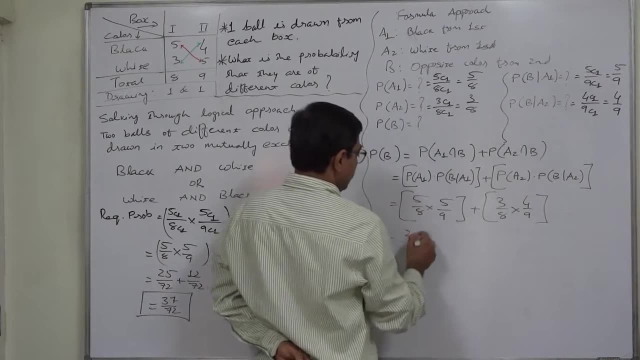 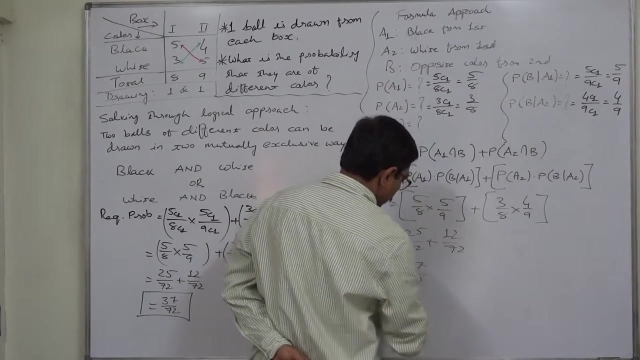 is 5 by 9 plus P of A2, is 3 by 8.. P of A1 is 3 by 8.. Into P of B, given A2 is 4 by 9.. 25 by 72 plus 12 by 72. So it comes to 37 by 72. But frankly, 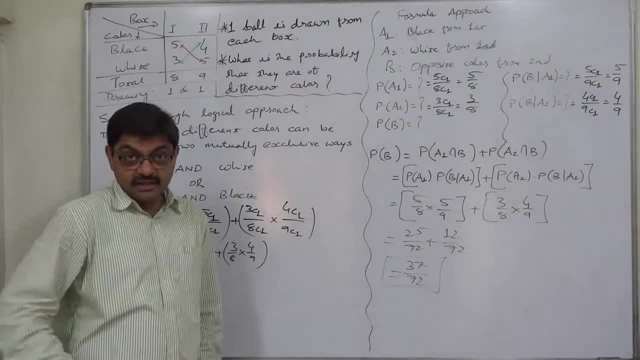 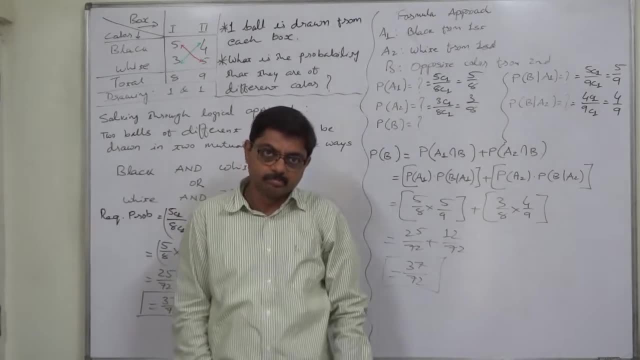 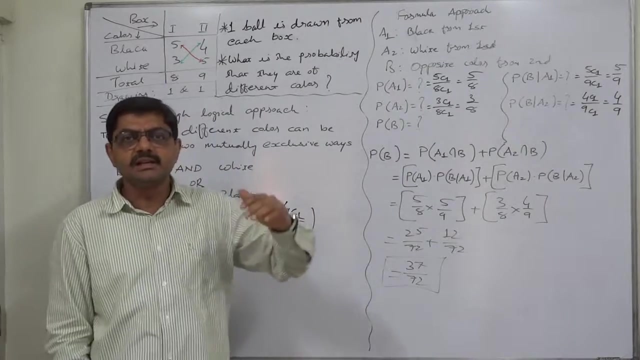 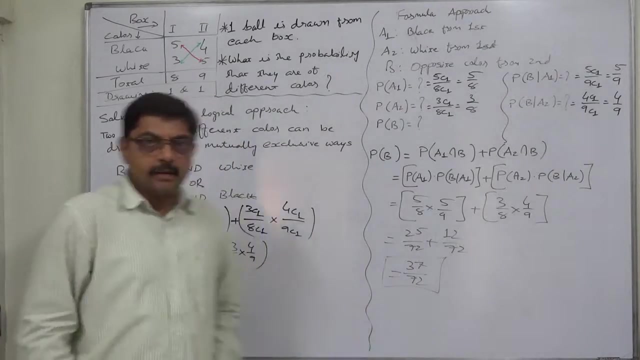 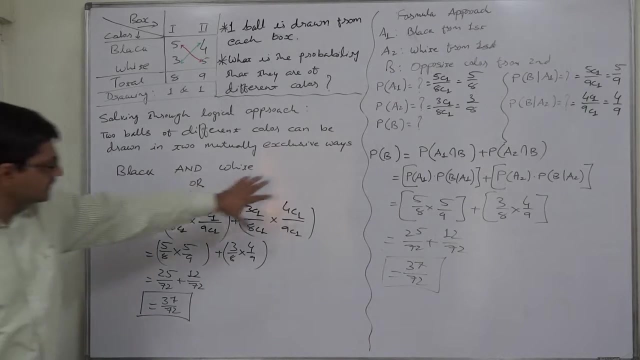 speaking. I may be criticized for my this statement, but this is not everybody's cup of tea. You can solve the problem in this way Only after reaching a certain level of understanding of various concepts and calculation of probability. But this is possible for a beginner in this chapter, Because in this approach we are using 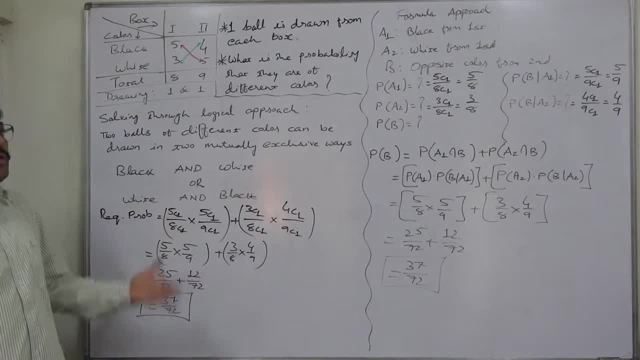 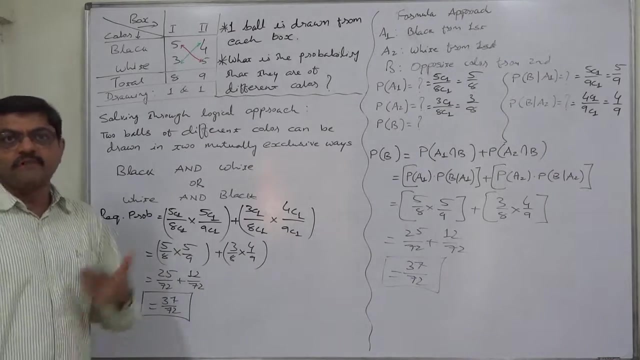 our common sense In which way? drawing a black ball from the first and white from the second, or drawing white from the first and white from the second, or drawing white from the first and white from the second. In this way, two balls of different color into consecutive.